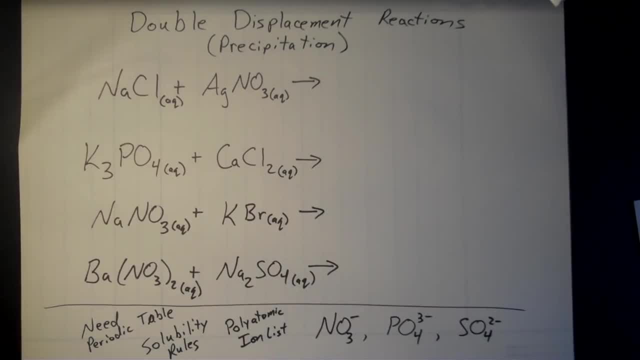 The next thing we're going to do is we're going to need a list of solubility rules, And the neat thing about these is the charges don't change during the course of this kind of a reaction. So whatever charge an atom has on the reactant side, it's going to have that same charge on the product side. In fact, we'll have to do that with the silver here in just a second. 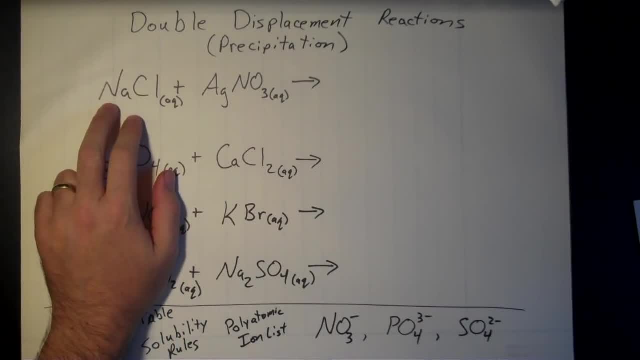 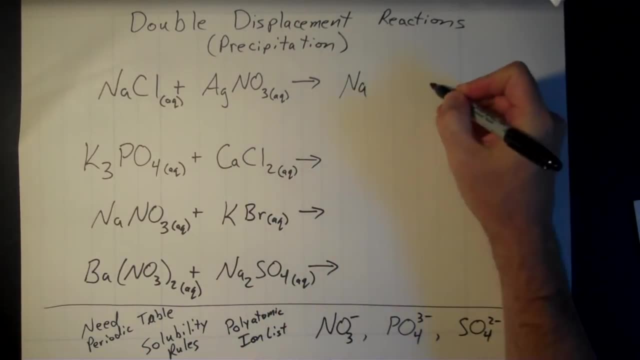 Alright. so let's go ahead and do this first reaction here. The way that I go about this is I'm going to bring just one of each ion over to the product side first. So I'm going to bring one sodium over, leave some space, put your plus sign for your other compound and put the silver with that. 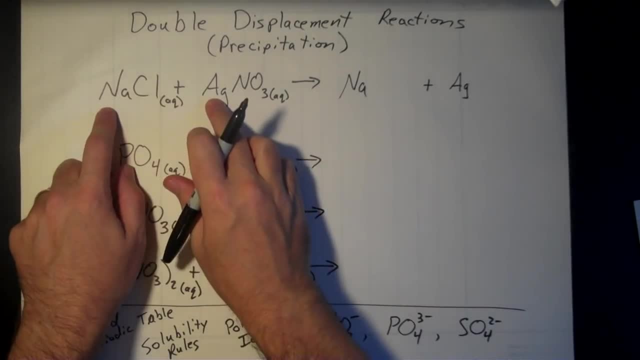 Just one of each cation. One of each cation, One of each positive ion. Of course there was only one on the reactant side, so not a big deal there, but we'll have to deal with that in some of these other ones. 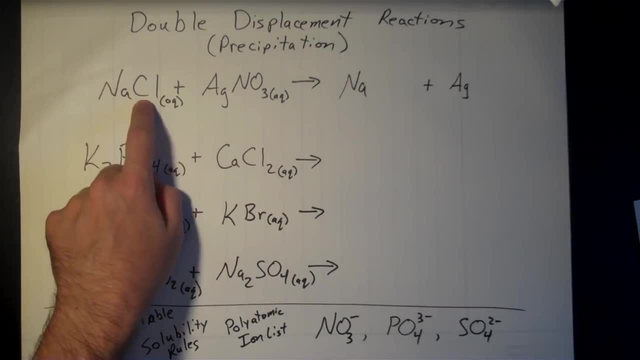 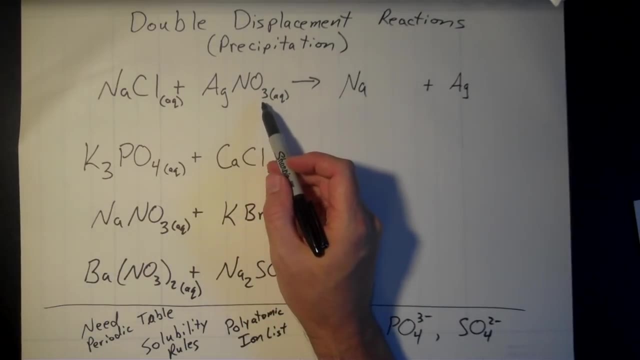 Then we're going to do the same thing with the anions: The chloride ion here, and the nitrate ion, the NO3.. And one thing I always tell my classes is that the only subscript you're automatically going to bring with it is if it's a part of a polyatomic ion like NO3 or the 4 here in PO4 or the 4 here in SO4.. That you'll come with it. Leave any other subscripts behind. 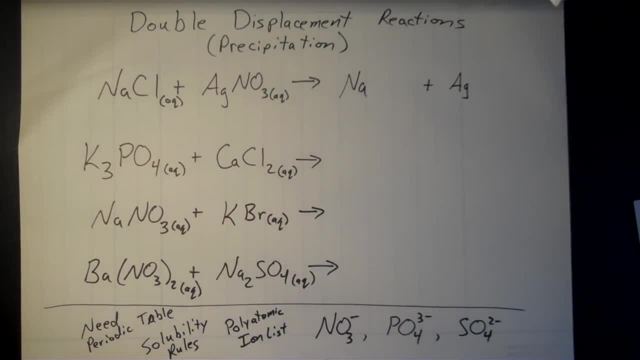 So for those. So I've got my sodium and my silver. I'm going to bring the chlorine and the nitrate over, but we're going to switch which cation they're with. So the chloride ion here is with the sodium. so on the product side I'm going to put that chloride with the silver, The nitrate ion here on the reactant side with silver it's going to go with the sodium on the product side. So there's my NO3 on the product side there. 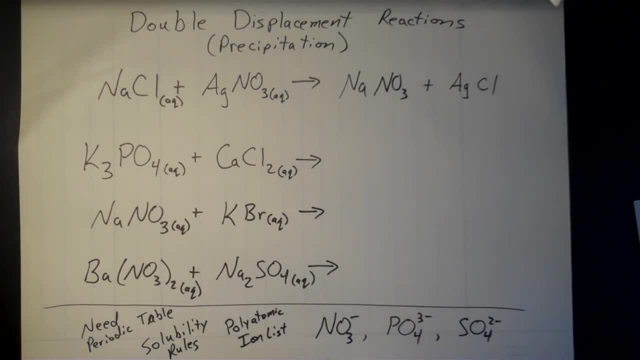 The next thing we need to do- and a lot of people forget to do this, especially on quizzes or exams- do this part. you need to balance out the positive and negative charge for each product substance. we need to make sure again, these are both ionic compounds. 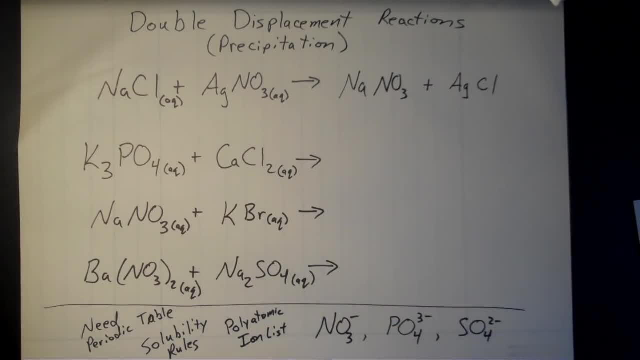 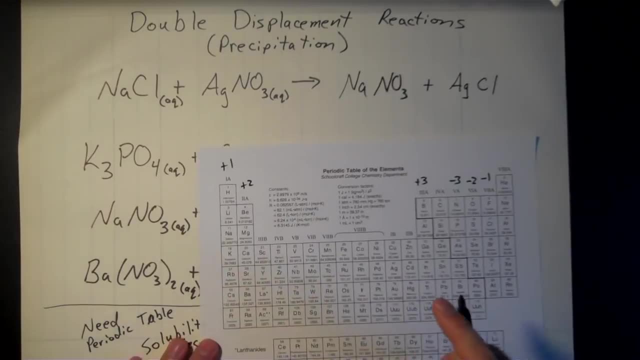 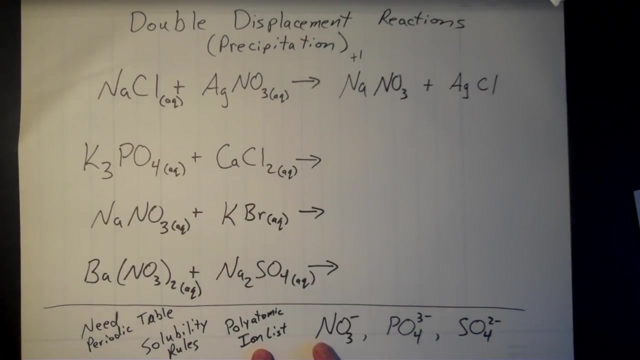 with any ionic compound, your positive and negative charges need to balance out. and so for the sodium, that one, we can figure out from its location in the periodic table here it is in column one. it's gonna have a plus one charge for that. and the nitrate ion, you can get that from your list of polyatomic ions. 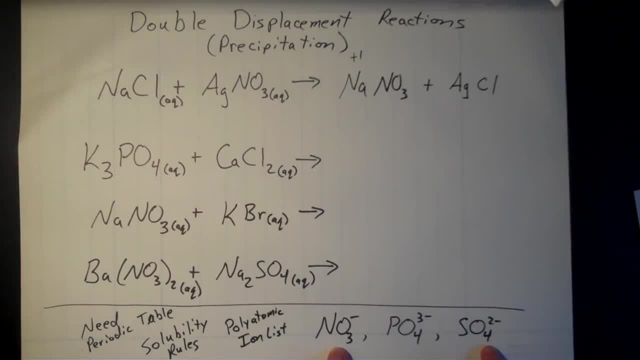 which I just have a very short list of them down here, just the ones that are in this particular, these examples that I'm looking at: there's my nitrate and it's got a negative one charge for that, and so if your positive and negative charges are the same, then you're done. you don't need to do anything else with that. 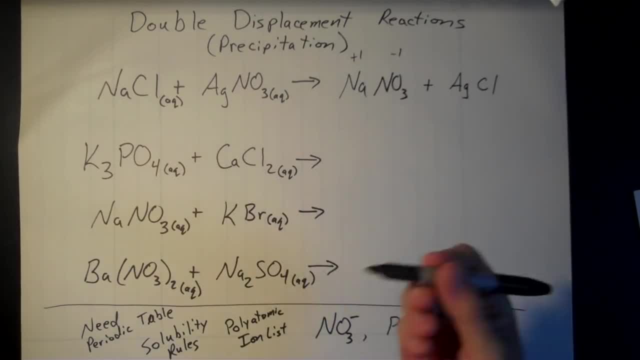 that's the correct formula. I usually go back and erase those. I'm using a sharpie here so I can't erase them. but there's my positive and negative charges. that and then the AG and the CL. let's start with the chloride ion, since we can. 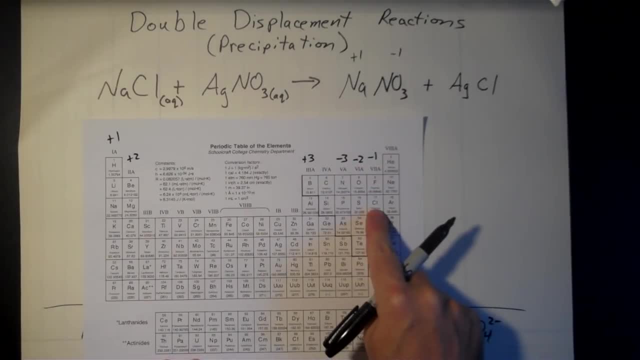 actually figure out that one from its location in the periodic table. it's in the second to last column. those all have a negative one charge, and then the H2O. and the H2O are the ones that are in the second to last column. those all have a negative one charge, and then the H2O are the ones that are in the second to last column. 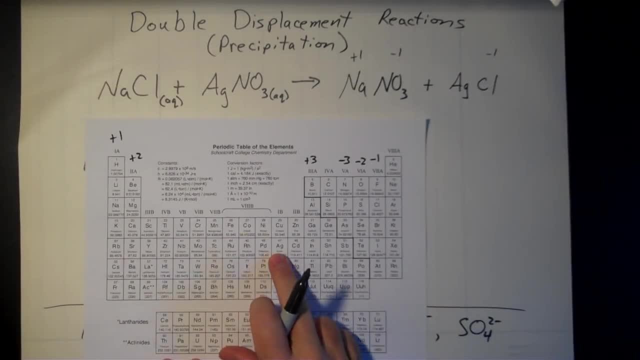 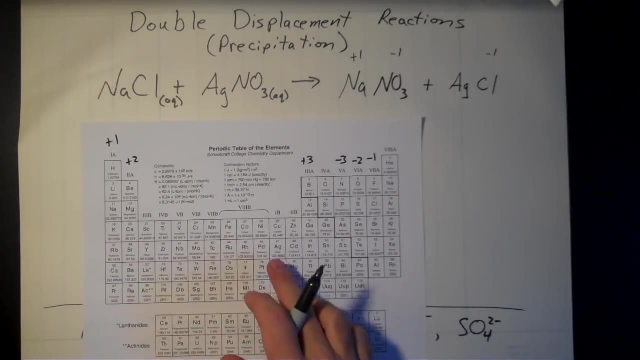 so we know chlorine is going to be a negative one for that. silver is over here in the transition elements and that one you can't tell based on its location in the periodic table, although you can memorize silver is always a plus one, but you don't have to memorize it for this one. here we can actually figure. 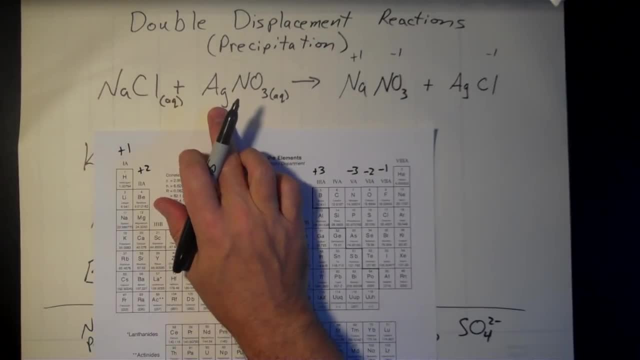 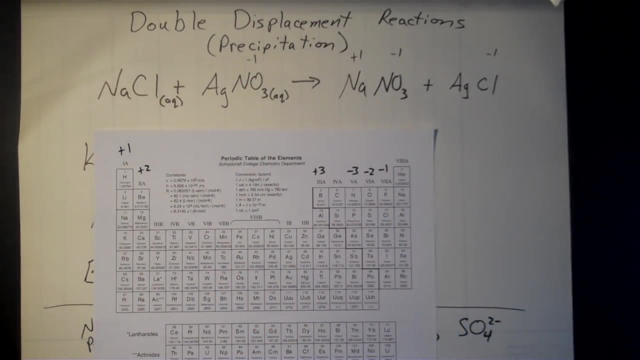 out what its charge is going to be on the product side, because it's going to be the same as the charge it had on the reactant side. it was with one nitrate ion on the reactant side which had a negative one charge, and so then, if we 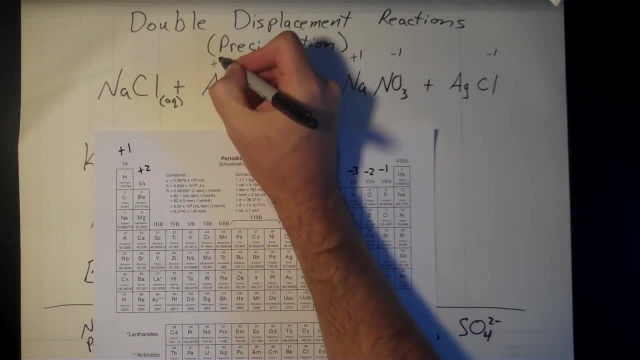 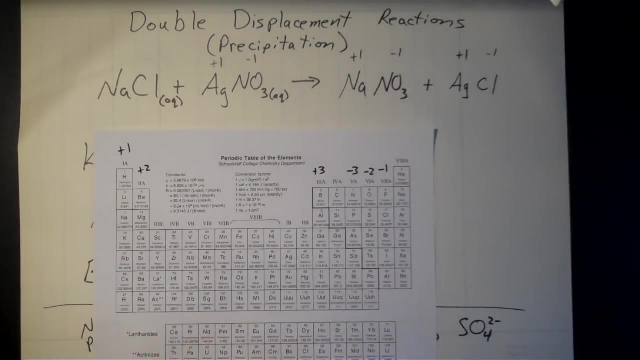 kind of work our way backwards here. silver then to balance that out, since there's only one silver, it's got to have a plus one charge. so if that silver is a plus one, then so is this one over here. you only have to do that for the transition elements, otherwise like. 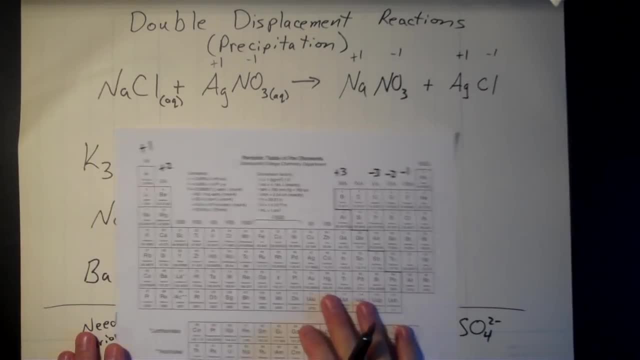 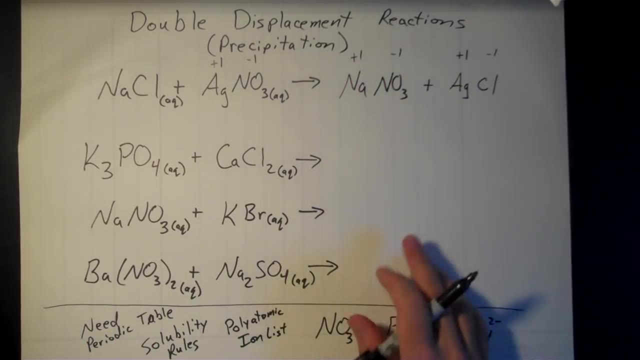 sodium or potassium or calcium- those you can figure out from their location in the periodic table. all right, so this turned out to be a really easy one, since all the charges were positive and negative. they have plus one, a negative one. they all balance out. we don't really have to do anything else as far as 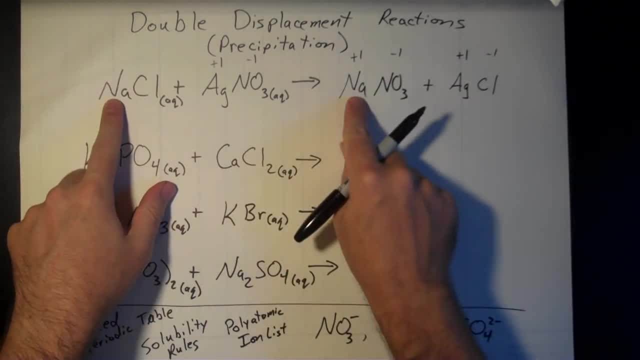 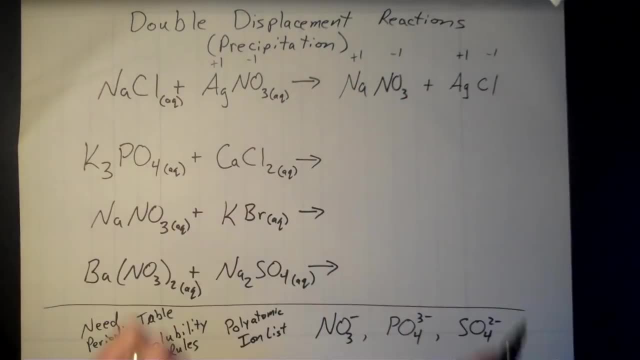 that's concerned, and in fact the whole equation is balanced. I've got one sodium, one sodium, one chlorine, one chlorine silver, silver and one nitrogen. three oxygens: one nitrogen, three oxygens where you can do that as one nitrate each, so that equation is already balanced. the last thing we need to do 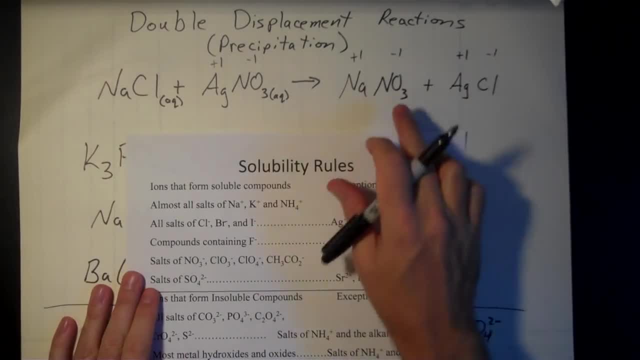 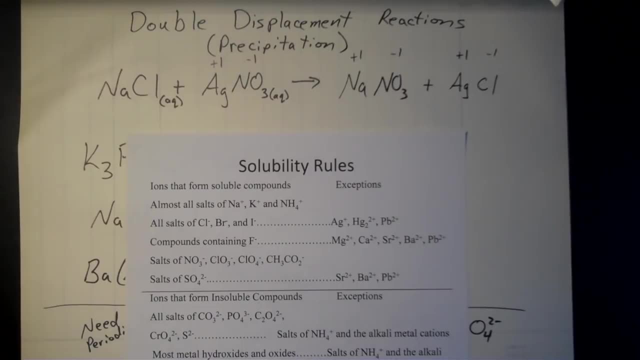 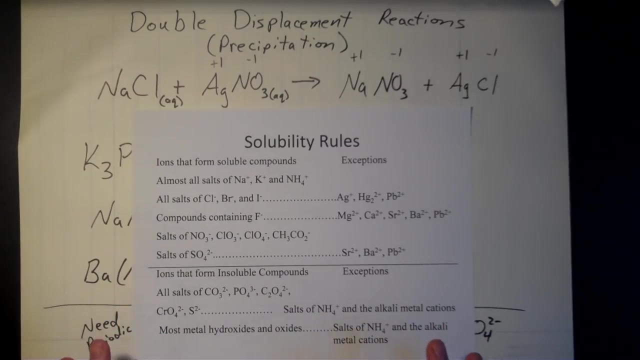 then, is to figure out which of our two products is going to be soluble or aqueous, and which one is going to be a solid or the precipitate from this reaction system, And so to do this, you'll have to use your solubility rules. so you want to have this. 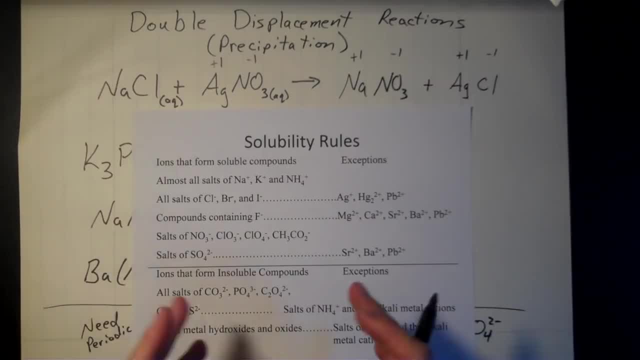 handy when you're doing these kinds of problems, And so your instructor may have you memorize these. some instructors give that to you, so it depends on who your instructor is, but you've got to have that list out and handy here. 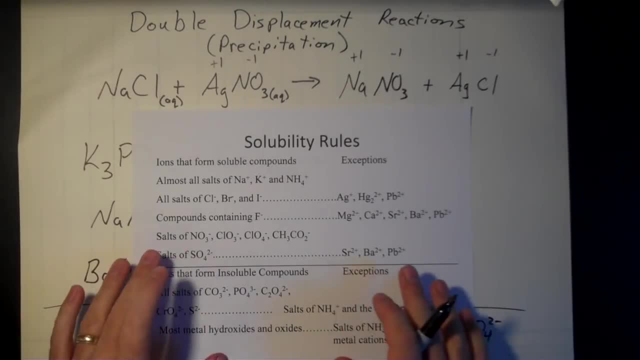 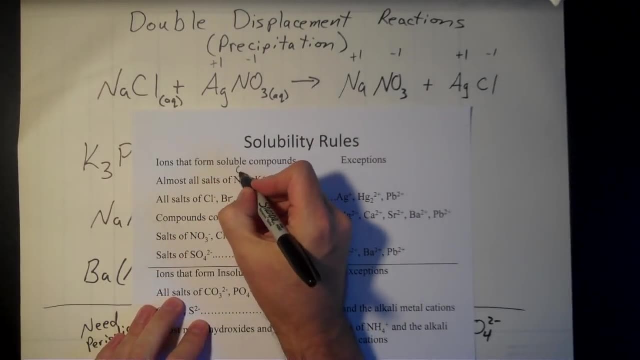 So the way I've got this- and every list of solubility rules can be a little bit different here. the way I've got this one set up is I've got soluble compounds up here, or ions that form soluble compounds. Again, these are going to be aqueous for us if it's soluble and then down here are ions. 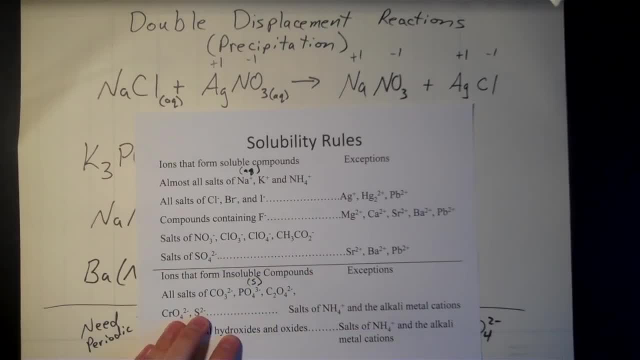 that form insoluble compounds. those are going to be solids, so we'll put a little S there for those. There are some exceptions to some of these ions, though, and so that's how we, that's typically how you'll see a solubility rule set up. 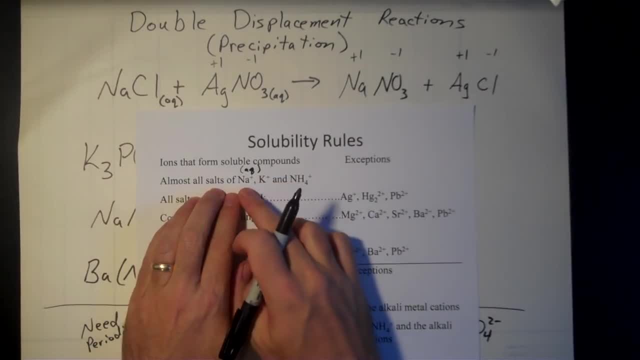 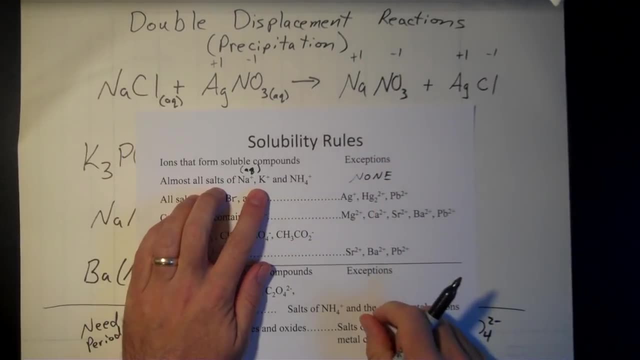 Notice, though, there's a few of these rules that don't have any exceptions, like sodium, potassium and ammonium salts, they're always aqueous, Okay, So there are no exceptions to that. Same thing for these ions down here. this is nitrate and chlorate and perchlorate, and 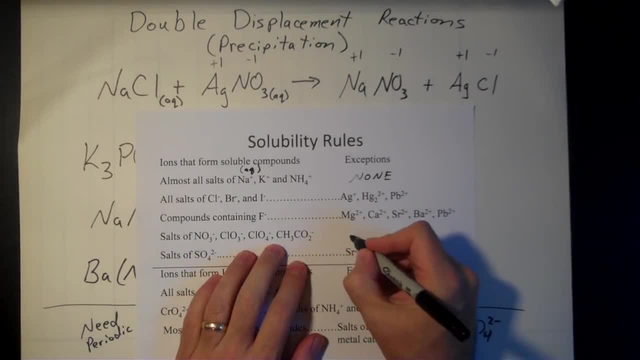 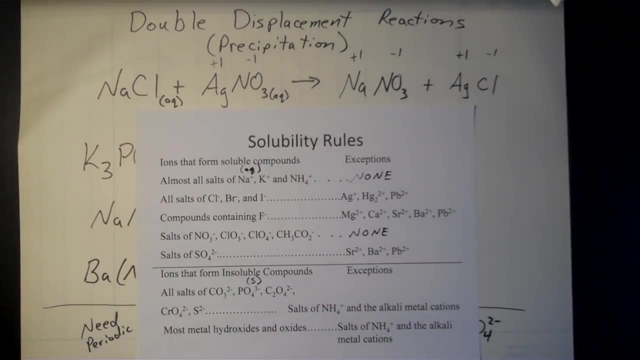 this is the acetate ion there. When those negative ions are in a compound, they're always aqueous as well. So there's no exceptions for those two ions, but there are for some of these other ones, so let's see if we come across any of those for this. 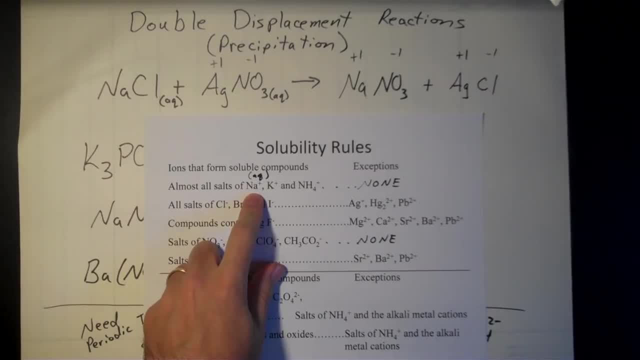 So let's start with sodium and nitrate and a good rule to memorize because it just shows up a lot of the time: Sodium is the rule for sodium and potassium and really it's all the alkali metals- I just put a few of them on here- and the ammonium ion. they're always aqueous, they're always. 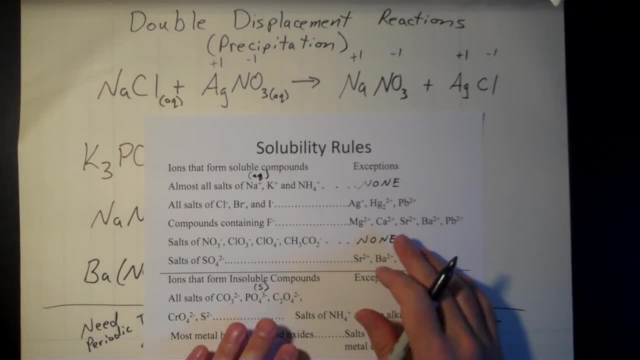 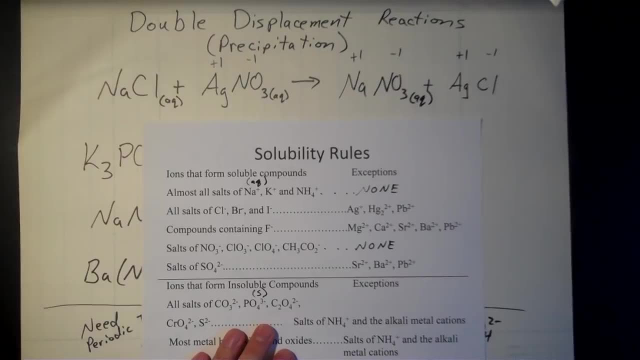 soluble. So if you see sodium in a compound, it's always going to be aqueous. you don't have to worry about what the other ion is that's with it, And so we can immediately put a little AQ then behind the NaNO3, because it's going. 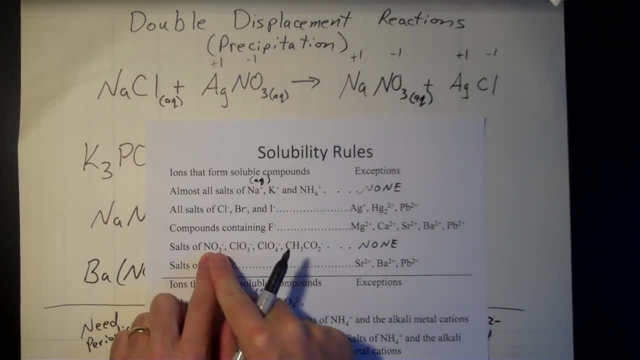 to be aqueous. We could also base this off of the nitrate ion, and it's got the same rule: Nitrates and all these other ions, they're always aqueous, they're always soluble. no exceptions there. So again, that tells us that's going to be aqueous. 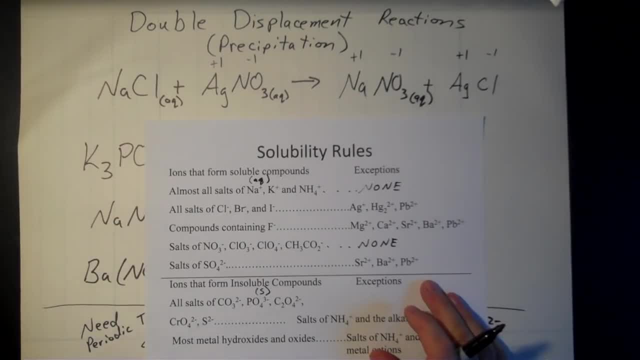 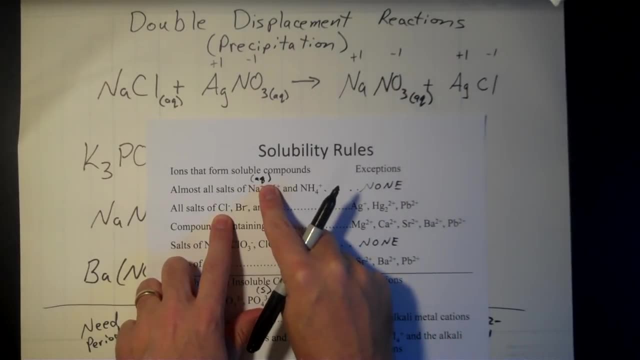 Then let's go with silver chloride and this particular list. I don't have a rule for silver, but I do have a rule for the chloride ion here, Cl- right here Chloride is usually aqueous, but there are some exceptions here. 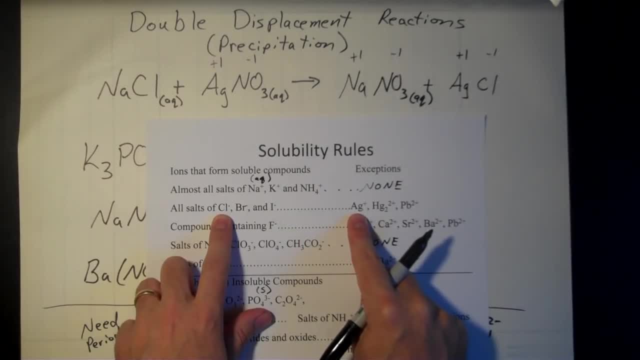 So that's when we have to look at the exceptions, and if you look at the first exception there, it's when chloride is with silver, and that's exactly what we have here, And so it doesn't follow the rule. The rule is that it's usually aqueous, but if it's an exception, then that means it's. 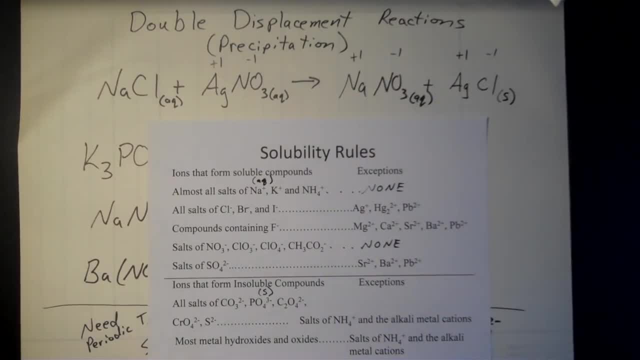 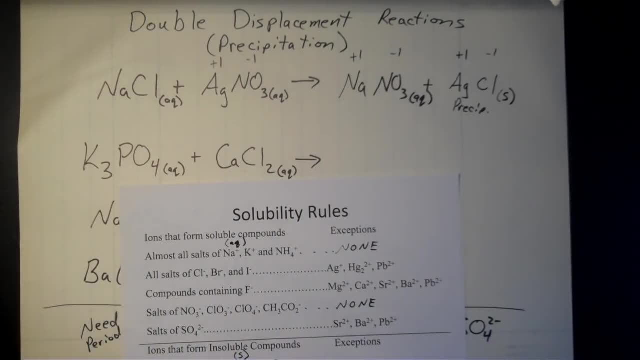 going to precipitate So that one's going to be a solid then. So that's our precipitate, So that'll be our precipitate That's going to form a solid. You'll actually see the solution turn cloudy and that's what your AgCl is then. is that? 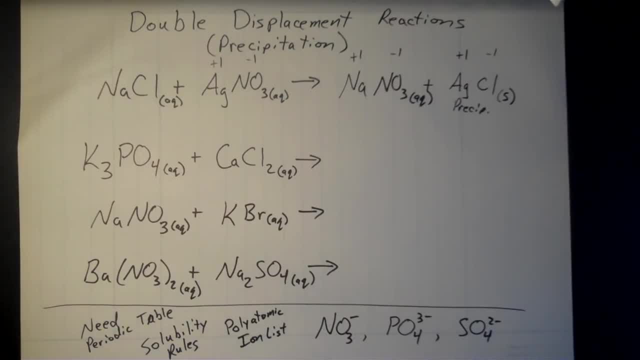 cloudiness. that's in there. All right, let's try the next one here. This one's a little bit tougher because some of the charges are different in this case, unlike the first one, where everything was a plus one and a negative one. 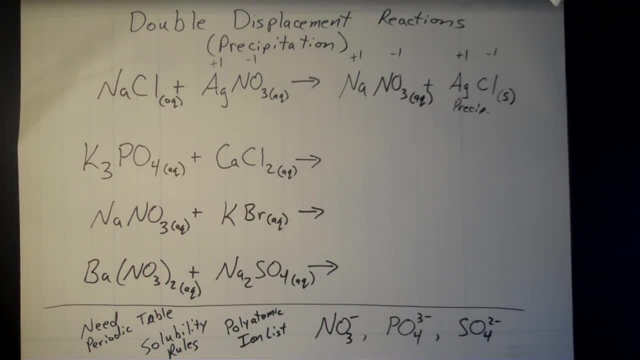 So for this one we've got K3PO4 and CaCl- Okay, CaCl2.. So again, we're going to start by bringing one of each ion over to the product side. The only subscript I'm going to bring is the four here. that's a part of that phosphate. 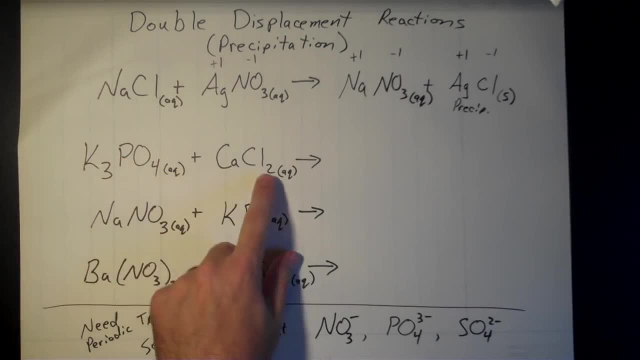 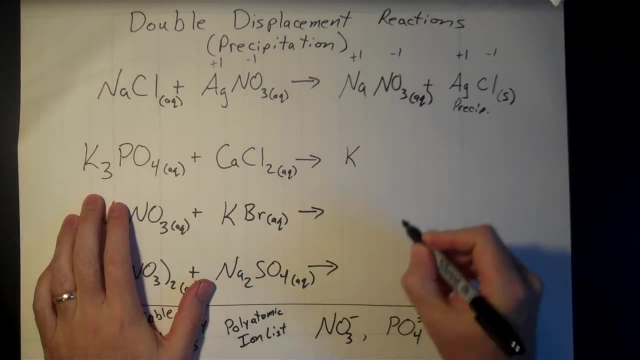 ion. The three here is just telling how many potassiums I have. The two here is telling how many chlorines I'm going to have. I'm going to leave those behind, So I'm just going to bring one potassium over to the product side and one calcium over to. 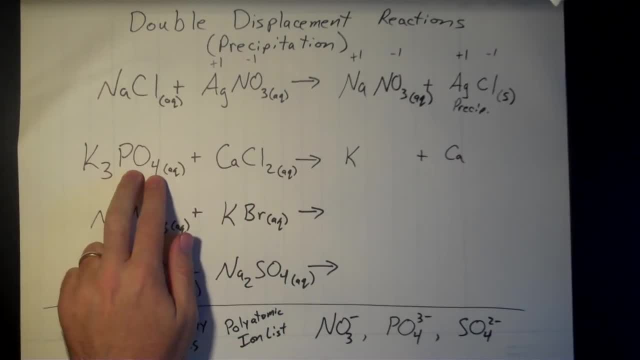 the product side, One PO4, but since it's with potassium on the reactant side, I'm going to put it with the calcium on the product side. there And again, there's two chlorines here. I'm only going to bring one of those over and that's going to go with the potassium. 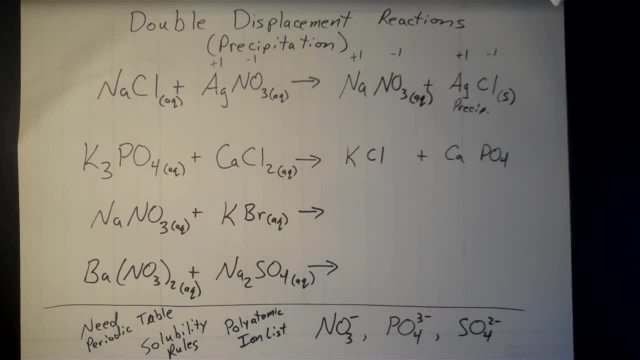 All right. So just figure out what your ions are and get them together Again. we're just switching which cation those anions are with, And so the potassium with the chlorine. here we can use the periodic table for this one. Potassium is in column one. 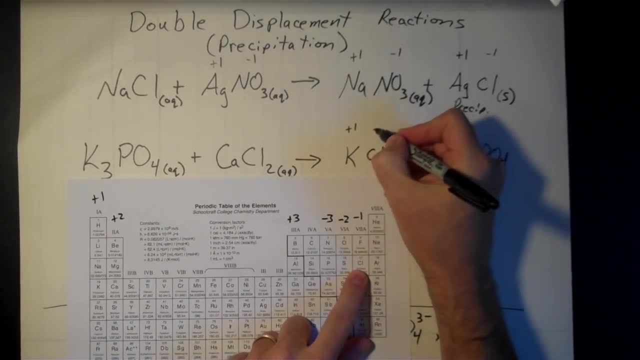 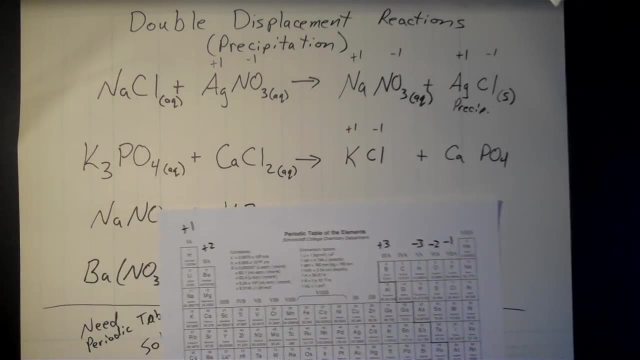 It's going to have a plus one charge. Chlorine is over here in the second to last column. It's got a negative one charge. Same positive and negative charge. That one's done. We don't need to do anything else with that. 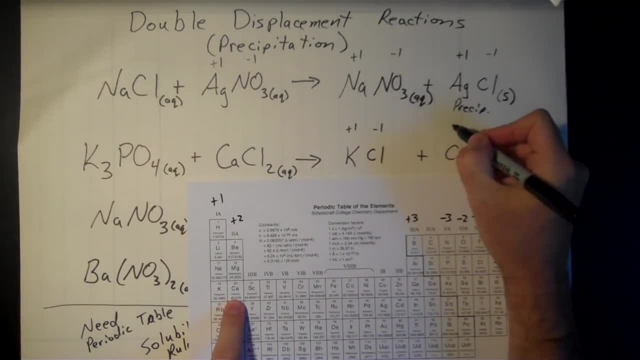 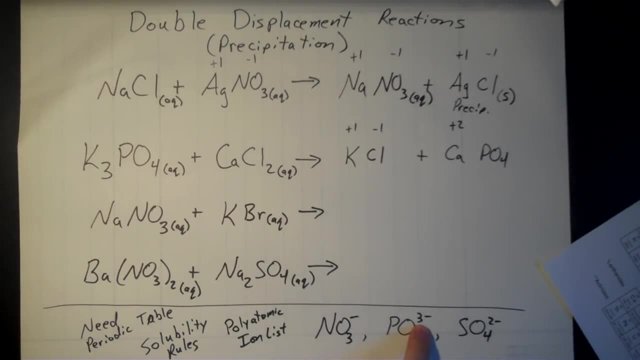 Calcium. on the other hand, it's got a plus two charge. It's here in column two or group two in the periodic table- Phosphate on our list of polyatomic ions. I wrote that down at the bottom here. It's going to have a negative three charge. 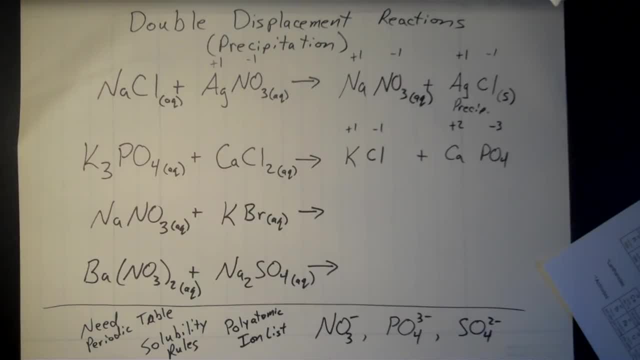 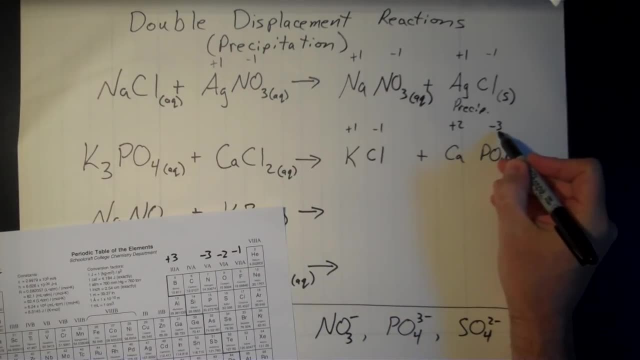 And so a negative three with a plus two. that's not balanced, as is. So we need more phosphates, We need more calciums, We need more of each of those. This is a great candidate For that little crisscross trick. 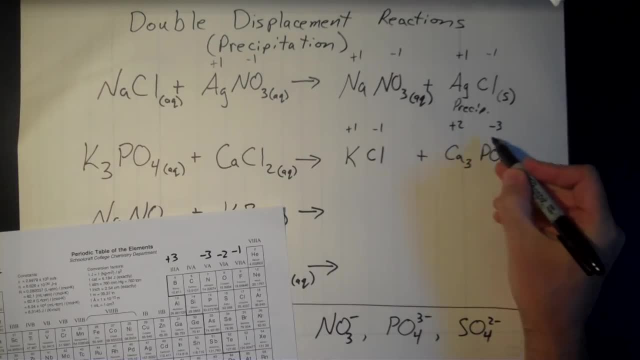 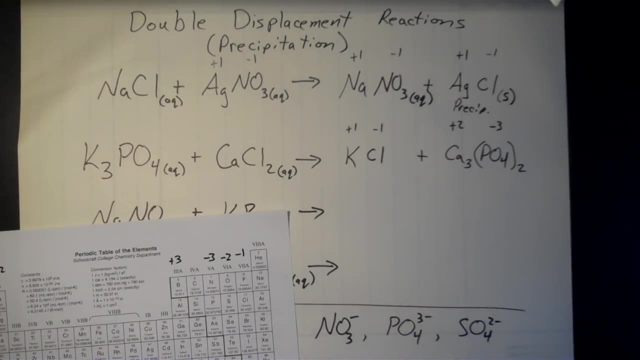 So I'm going to cross this over. I need three calciums and take the two here. That's how many phosphates? since I have more than one polyatomic ion, I need to put it inside of parentheses and we'll put the two outside of it. 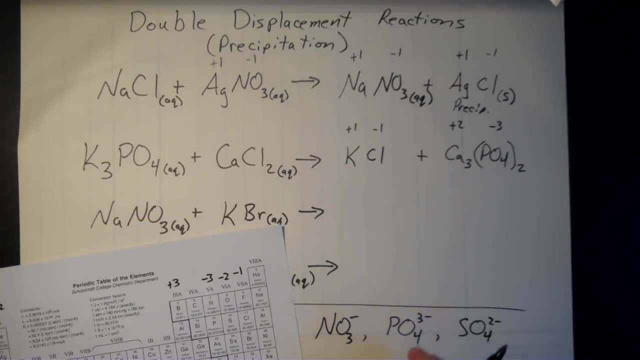 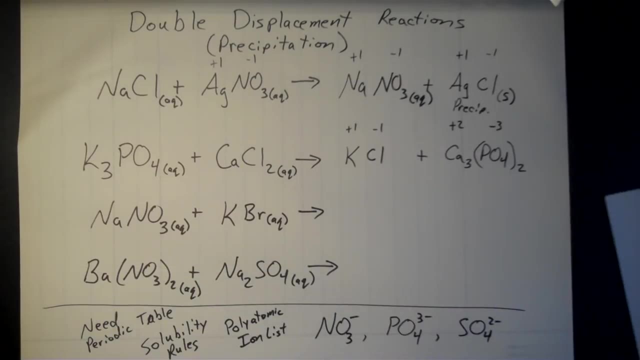 Otherwise it looks like you got 42 oxygens there. All right. So we want four- or I'm sorry, two- PO4 ions for that, All right. So now each of those formulas is balanced. We don't need the periodic table anymore. 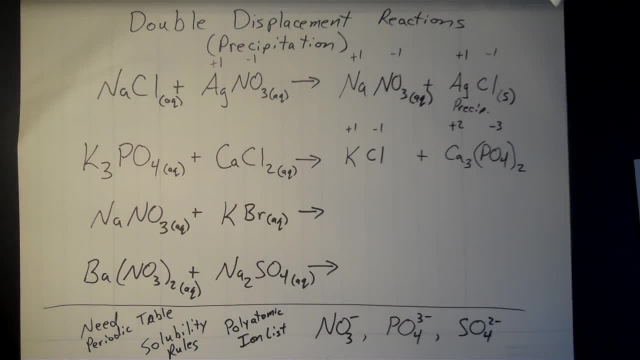 Now we can balance the equation Uh for this particular Particular system, and we could start with the um, with the potassium here. I've got three here and only one there, So I can put a three out in front of that uh, but I may need to do some other things. 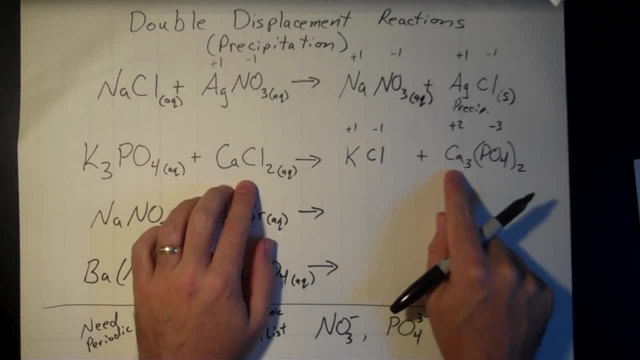 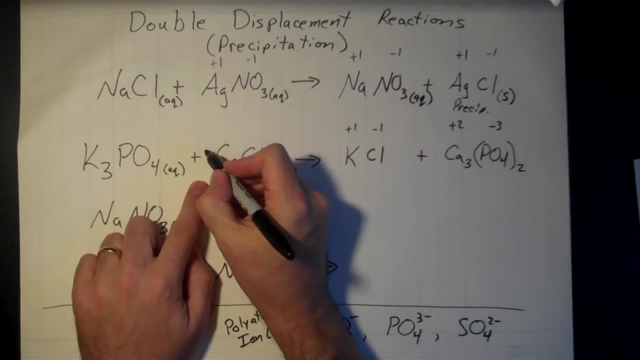 here as well, Uh, and so let me go, let me. I'm going to start with the calcium in this case. I've got one calcium here and there's three of them, uh, over here, And so I need to put a three out in front of the CACL2 to balance that part out. 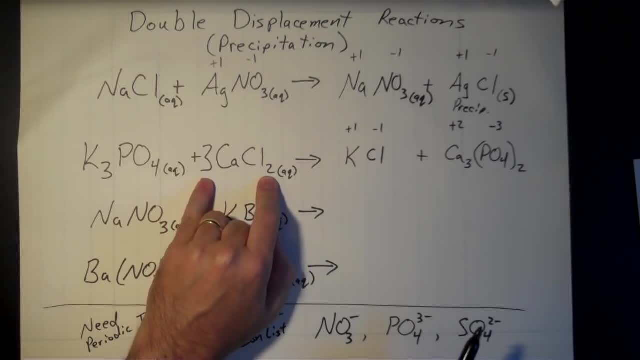 Uh, and now that's going to give me six Chlorines. three times two is six chlorines. I've only got one on this side, So I need to put a six out in front. Can you see why I didn't want to put that three there? because I was kind of looking. 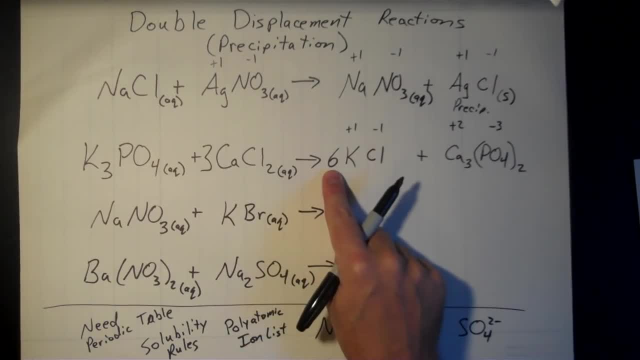 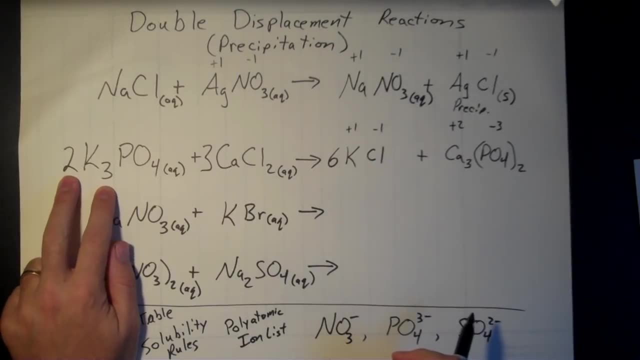 ahead there. I figured I wouldn't need that, Uh, and so now that gives me six potassiums for this, I can go back over here. I've only got three. at this point I need to put a two out in front of that. 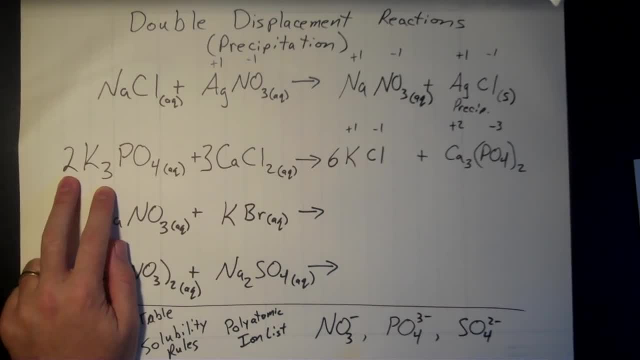 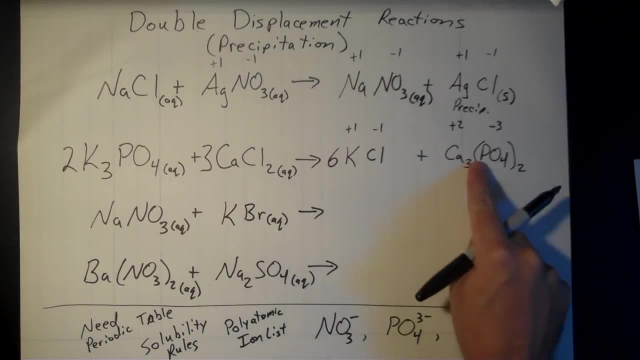 That'll give me my six potassiums now to match up the six potassiums that I have there. Notice now, that gives me two phosphorous and eight oxygen, And that matches exactly what I have. Okay, So over here, two phosphorous and two times four is eight oxygens there. 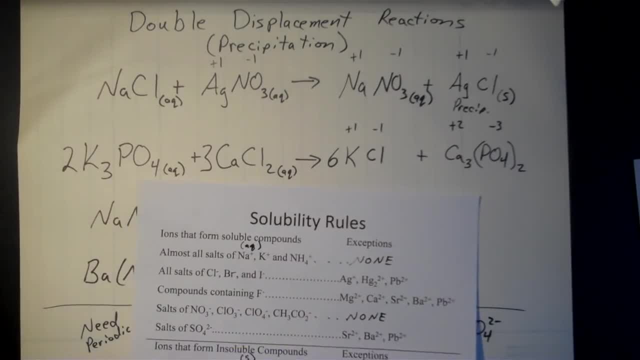 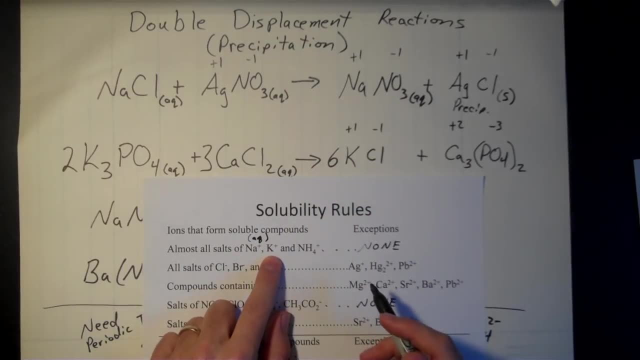 All right, So that's balanced. Uh, there's our balanced equation. Last thing we need to do: bring in the solubility rules and go through those. And here's CACL. And again, a good rule to know off the top of your head is that potassium salts- they're 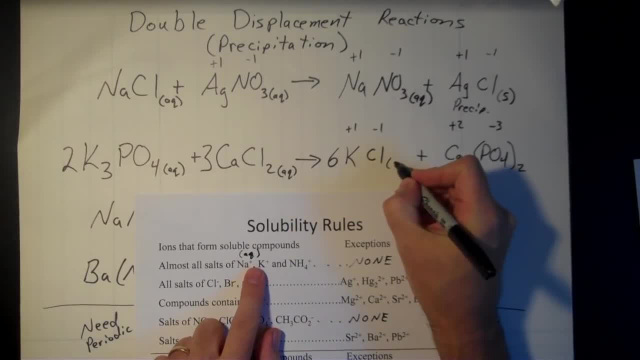 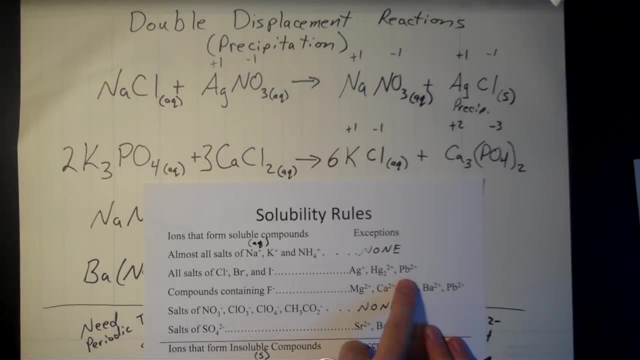 always aqueous, They're always soluble- No exceptions to that- And so we can put a little AQ in there. We could also go with the chloride rule there. They're usually aqueous and potassium, you notice, is not one of the exceptions. 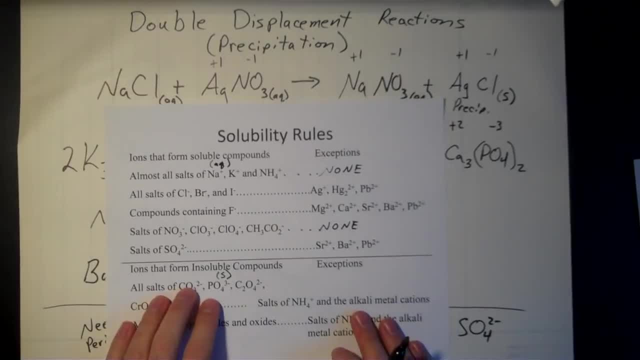 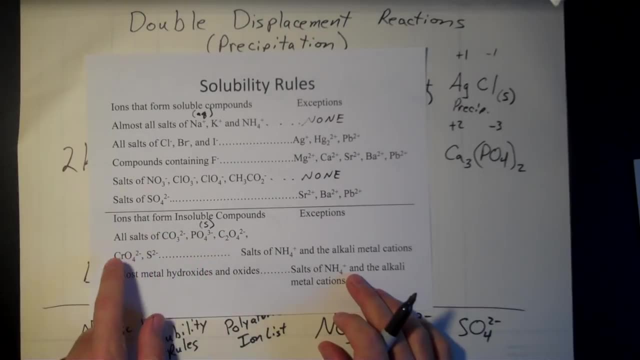 So it just follows the rule. It is aqueous there, And then down at the bottom of our list, we got to look at calcium versus phosphate, Uh, and down here I've got salts of carbonate, phosphate, oxalate, chromate, uh and sulfide. 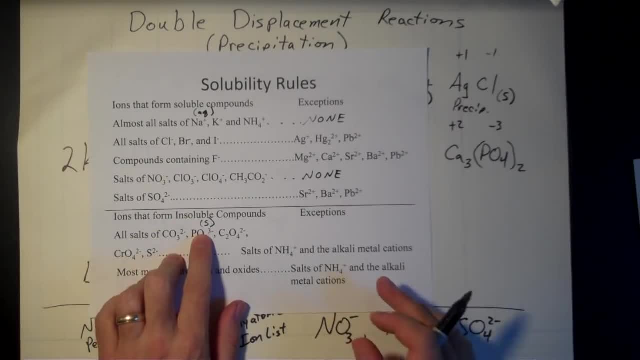 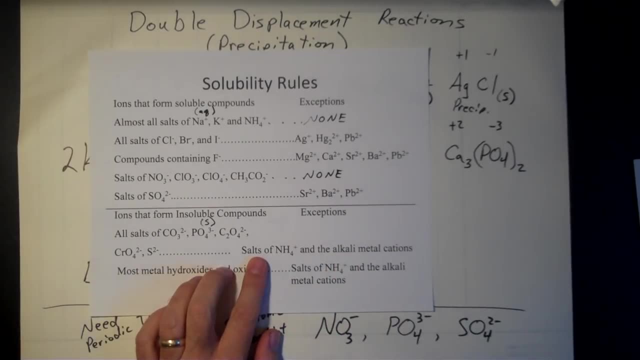 ion. They're, uh, they're usually solids, They're insoluble, They're going to be our precipitate. The only exceptions here are the ammonium ion and the alkali metals, That's that column one, lithium, sodium, potassium, rubidium, cesium, francium, uh, francium doesn't. 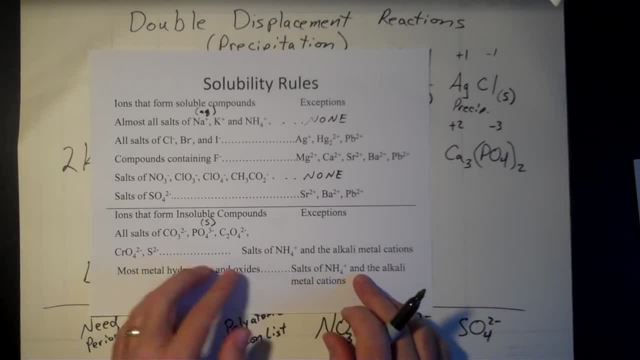 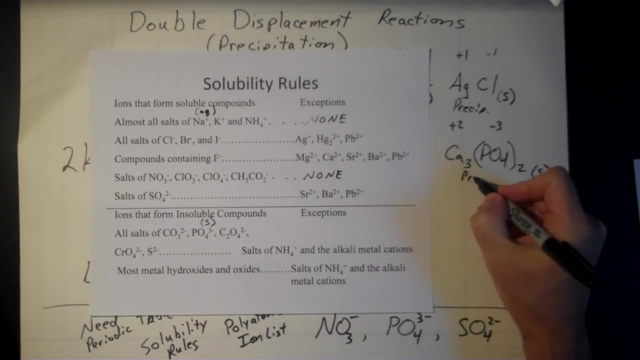 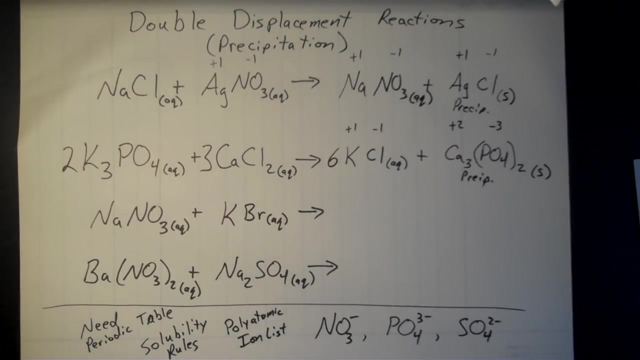 do anything, And so the calcium ion there, uh, is not one of the exceptions. So that should precipitate. That's going to be our solid then for this one, That's our precipitate, All right, And so, again, that's how we use the solubility rules. 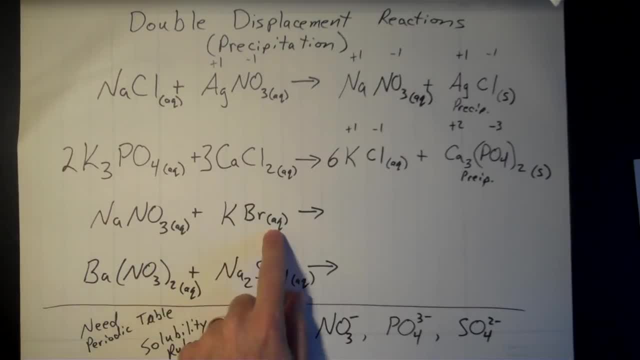 All right, Let's try this one. Uh, we've got sodium nitrate and potassium bromide. We'll do the same thing: Bring one sodium over to the product side, one potassium over to the product side. We're going to switch those ions. 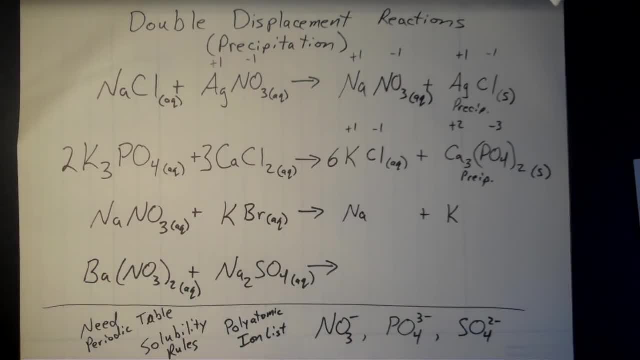 The three. here is a part of the polyatomic ion, like I have down here, So I'm going to leave that together. That's going to go with the potassium ion, the bromide ion. I'm going to switch that over. That's going to go with the sodium, and we can balance out our positive and negative. 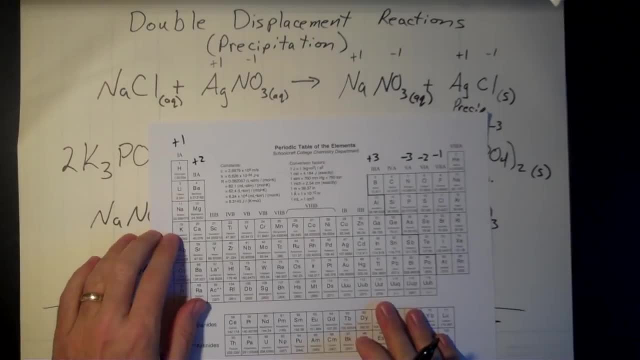 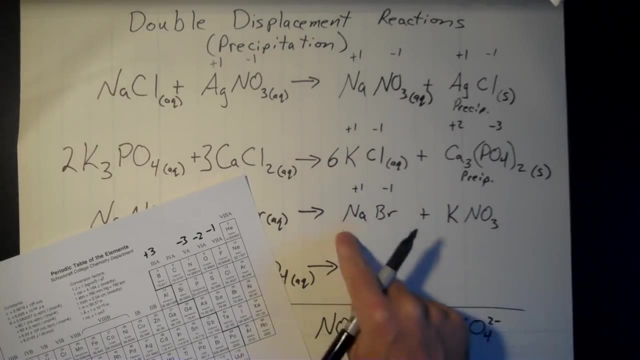 charges. Here's our periodic table once again. And so what do we need? Sodium and bromide. Here's sodium in the first column, plus one bromide ion in that second to last column is a negative one plus one and negative one. 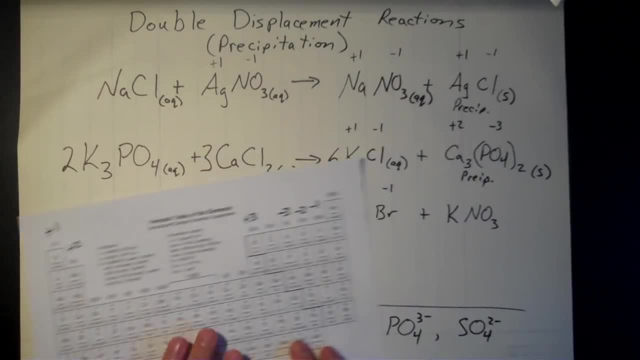 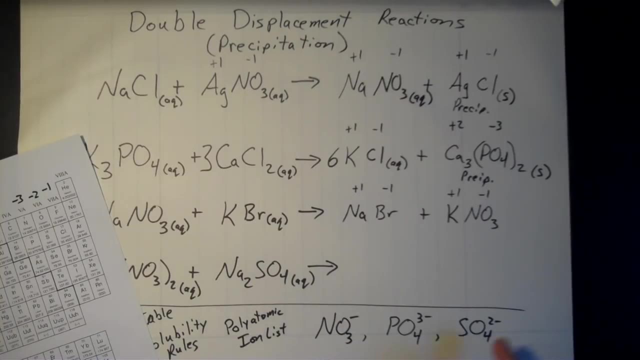 That formula is already balanced. Potassium also is in column one. here It's a plus one, And down here at the bottom I had nitrate ion. That one's a negative one, That one's all set to go as well. So that whole equation is balanced. 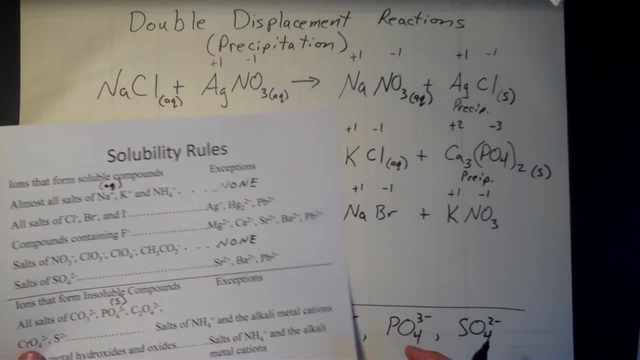 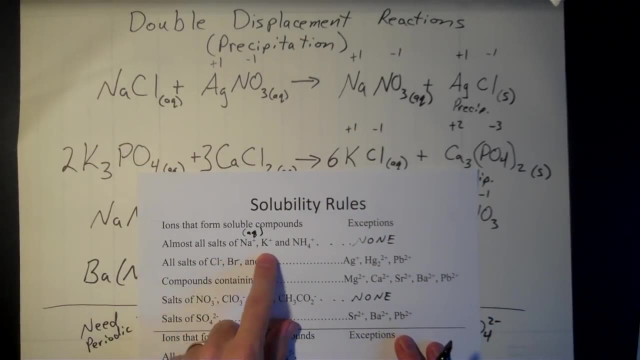 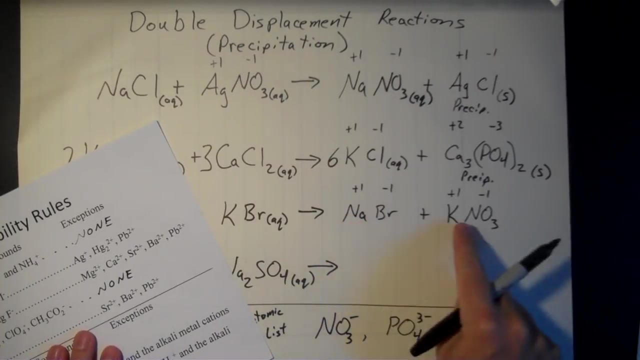 So we got sodium with bromide, potassium with nitrate. Now we're ready. This is going fast, isn't it? We need the polyatomic ion list, and actually we can figure everything out from this first rule. here, with no exceptions, All sodium salts, all potassium salts are aqueous, and that applies to both of our substances. 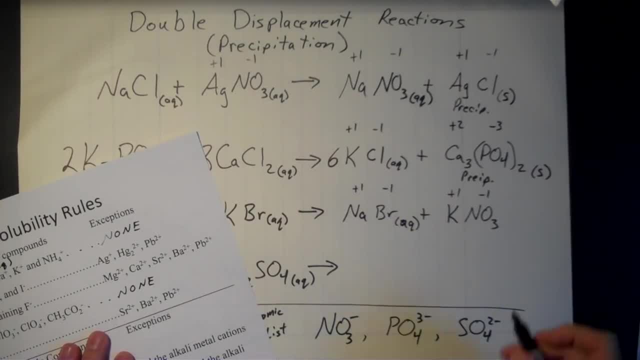 here And so, oops, I need an AQ there because sodium bromide is aqueous and I need an AQ there. I need an AQ there because potassium nitrate is aqueous. When both of your products are aqueous, you can just cross those off and write no reaction. 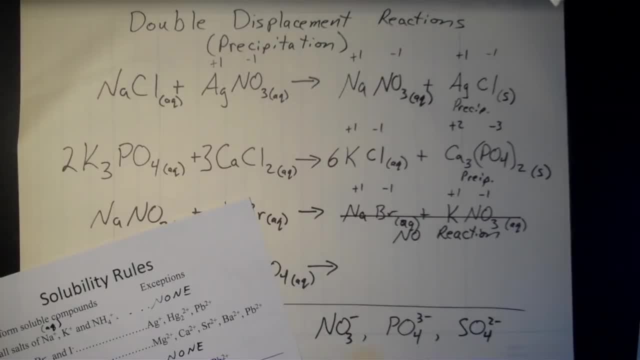 If you figure that out right off the bat, then you're ahead of the game there. But sometimes you got to figure out what ions you're putting together before you can make that decision. So if both your reactants are aqueous and both of your products are aqueous, usually, 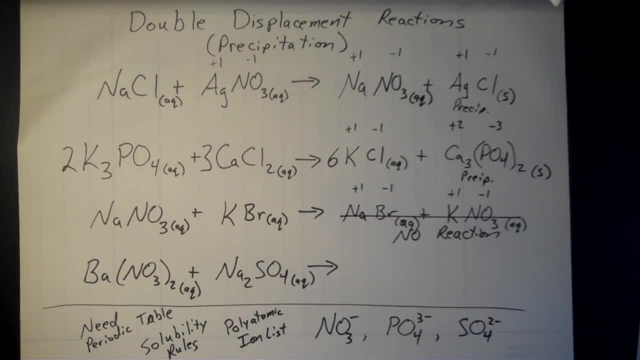 that's going to be a no reaction, then for that, All right, Let's try this last one. We've got barium ion with nitrate and sodium ion with sulfate. Again, we want to bring just one of each of those, So we're going to leave behind some of these subscripts. 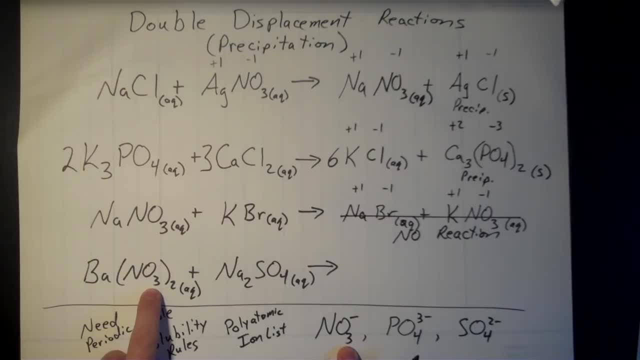 The only subscripts we're going to bring are those that are a part of the polyatomic ion, like the three in nitrate or the four in sulfate ion. So we'll bring over one barium- leave some space there- and one sodium- Yes, there was two here, but I'm only going to bring one of those over for that. 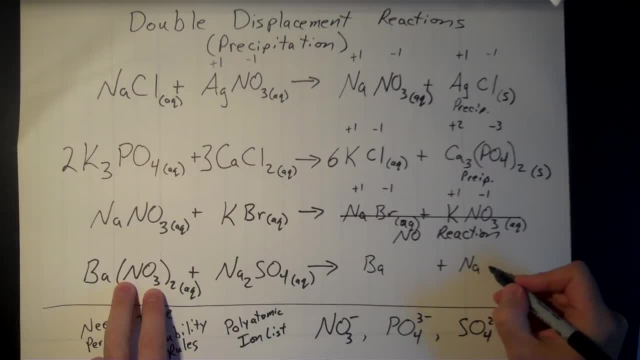 And then the NO3, we're going to leave behind the subscript two. The NO3 is going to go with the sodium, so we'll put NO3 there And the SO4 that was with the sodium. that's what we're going to put with the barium ion. 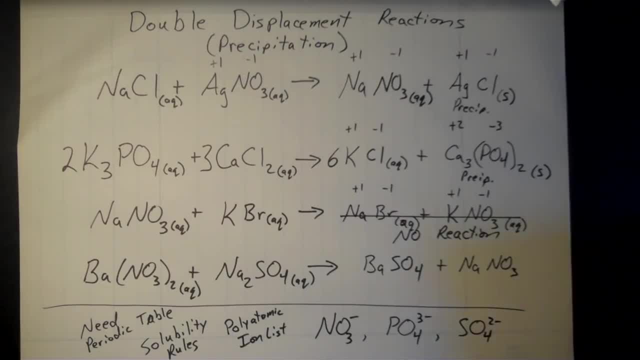 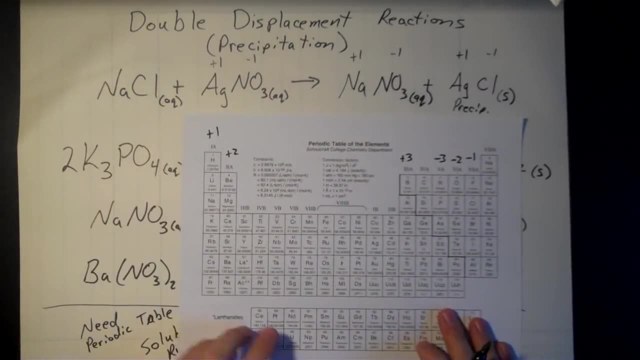 there All right. Now we need to balance out those positive and negative charges. so back to the periodic table Again. you got to have all this stuff handy when you're doing these things. And so for barium with sulfate barium is in the second column here, way down near the. 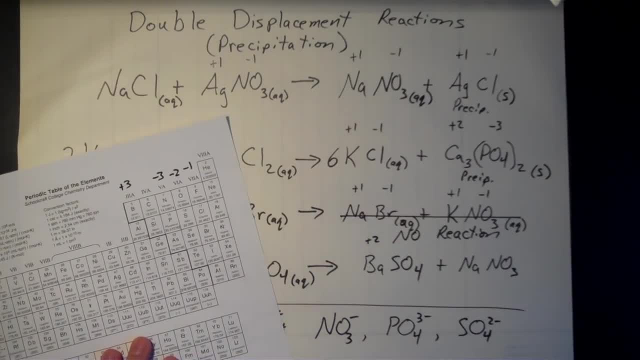 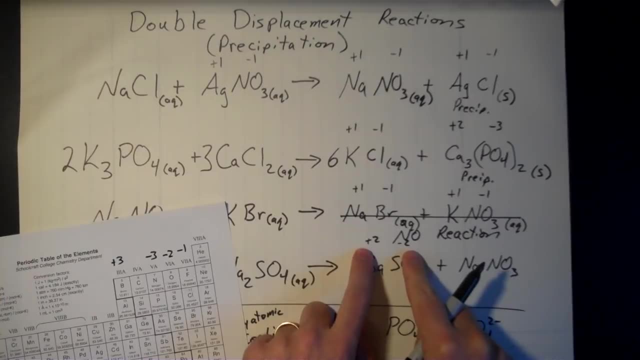 bottom and that's a plus two charge. so I got a plus two there. for barium Sulfate ion. I wrote it down at the bottom here. It's a negative two, so negative two there. I've got the same positive and negative charge there. 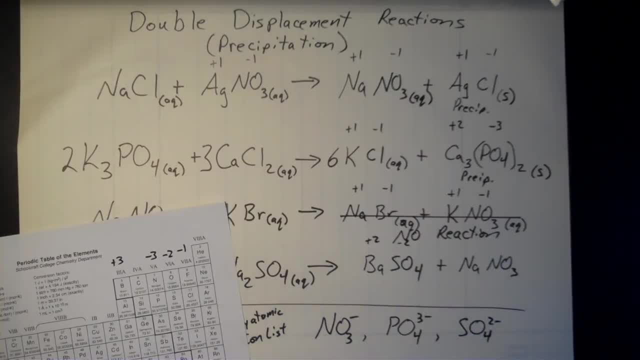 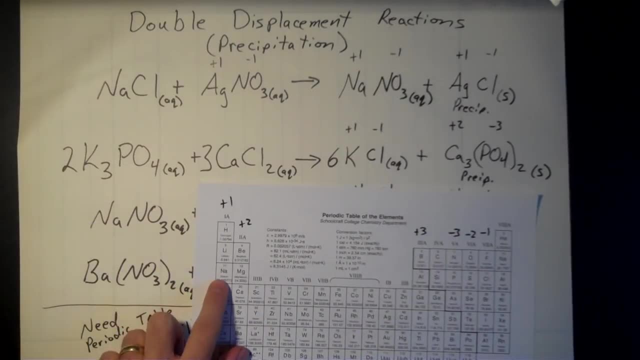 I don't need to do anything. Don't crisscross that, because you've already got the same positive and negative charge. It's already in its simplest form, so that one's done Sodium with nitrate, again sodium. you start memorizing these after a while, just kind of. 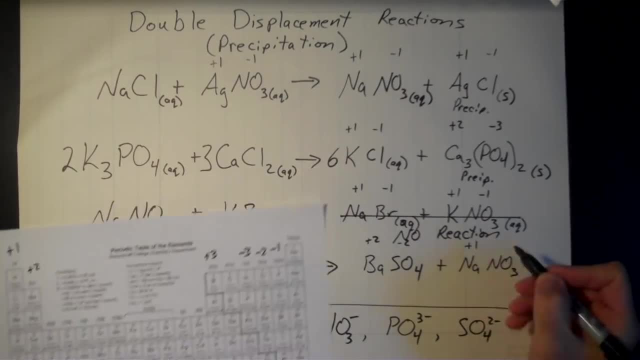 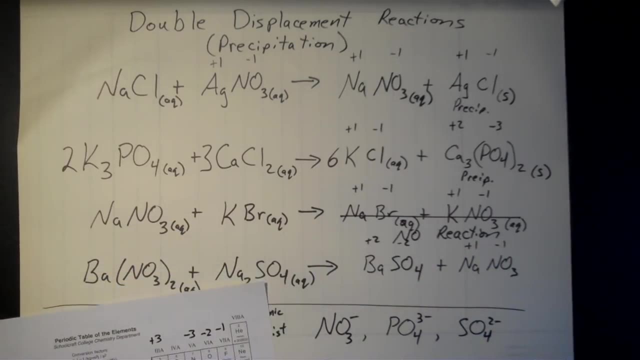 by default, not on purpose. But sodium is a plus one and nitrate ion here is a negative one charge. so same positive and negative charge there. That one's all set as well. Now we can balance the equation. I have one barium, one barium. 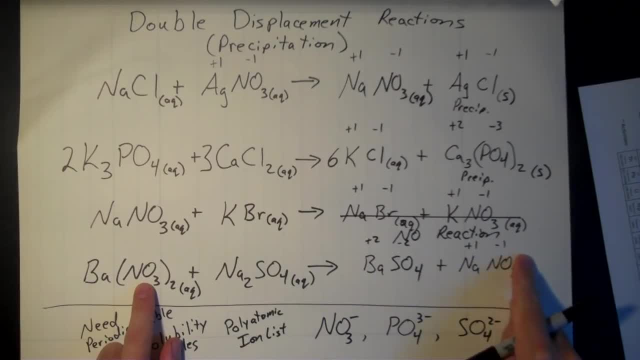 I have two NO3 groups here, but only one NO3 group on the product side, so I need a two out in front of that. And then I've got two sodiums there. Hey look, putting the two in front balances out the sodium, so we don't need to do anything. 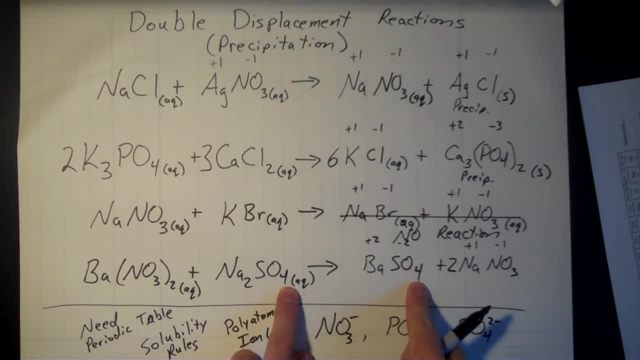 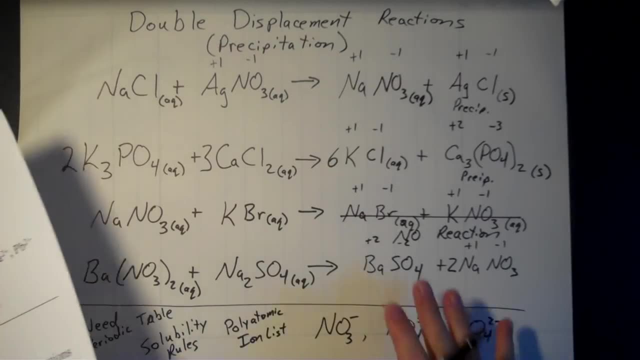 else there And I've got one sulfur and four more oxygens. one sulfur and four more oxygens there. That's balanced. then, just by putting that two out in front, All right, so the equation's balanced. Last thing we need to do. 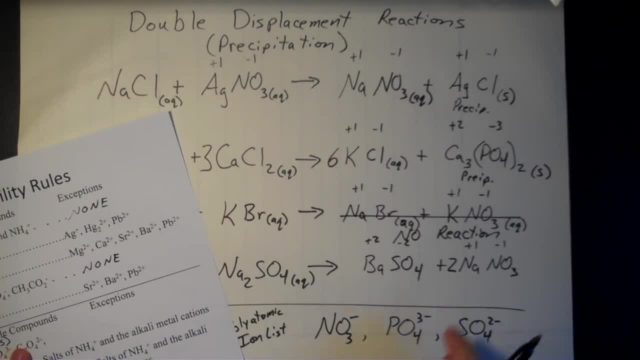 Bring back the solubility rules. Can you figure out which one of these is already going to be aqueous? There's our sodium salt again. So if you see sodium in a compound, you can pretty much automatically write that AQ in there. 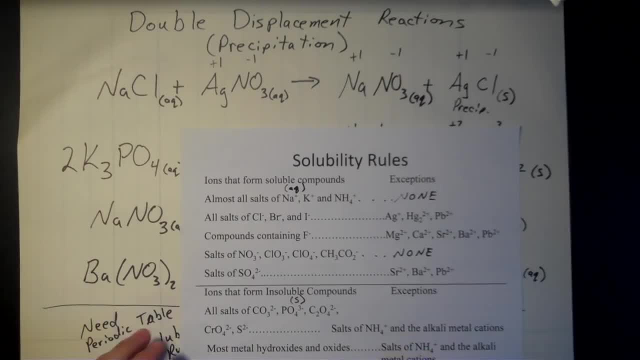 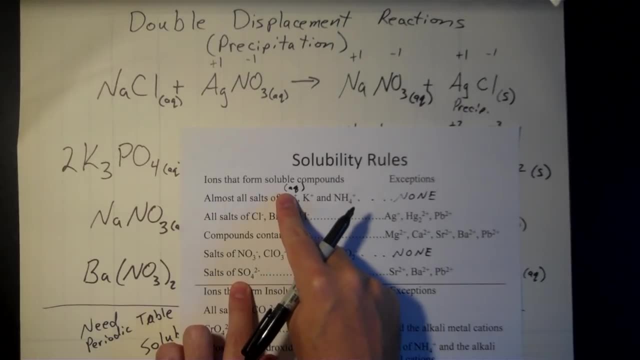 That lets you focus in on the other substance there, the BASO4.. And so let's find sulfate ion. Here's sulfate ion. Sulfate is under our usually aqueous substances, here soluble aqueous. same thing there, But there are some exceptions. 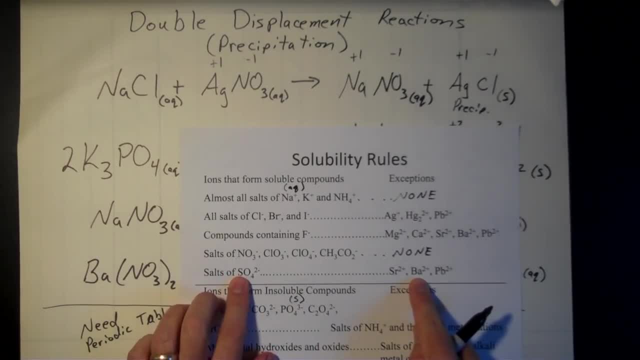 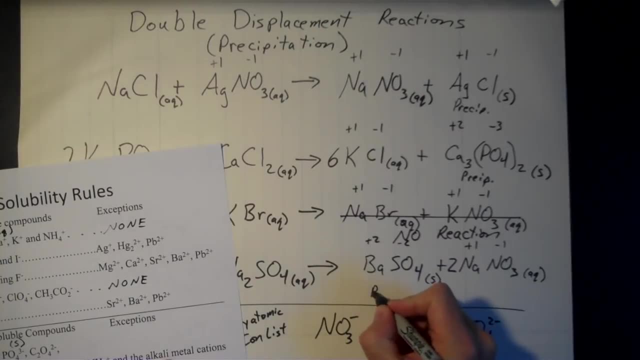 And that second exception: in barium ion, Sulfate ion should be a precipitate. then It does not follow the rule for sulfates. So barium ion with sulfate, that's going to be your precipitate. So again it doesn't. it's not always the first or the second in there. 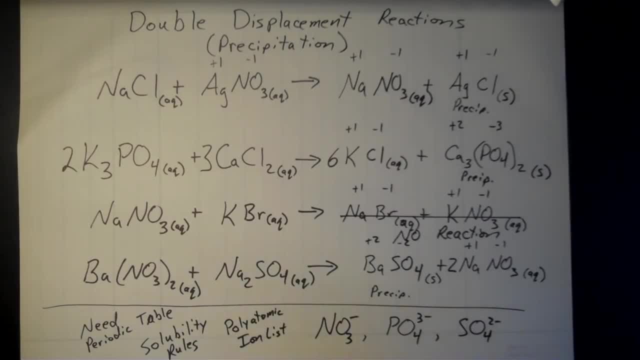 Again. hopefully you see that from this. That's how you complete double displacement reactions.